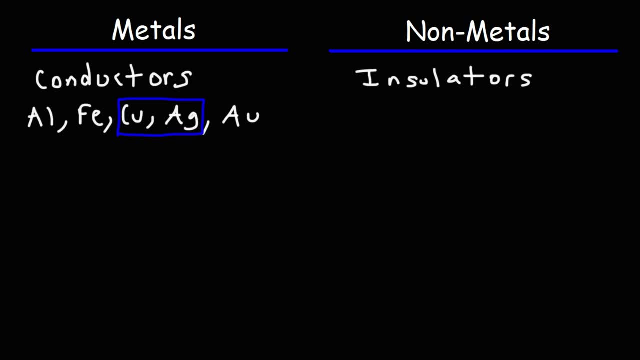 very good conductors of electricity, Even gold as well, but gold is expensive. Examples of non-metals include oxygen gas, the air that we breathe, nitrogen gas, which makes up most of atmospheric air. About 79% of the air is nitrogen, about 20% is oxygen Chlorine. that's a non-metal. it doesn't conduct electricity. 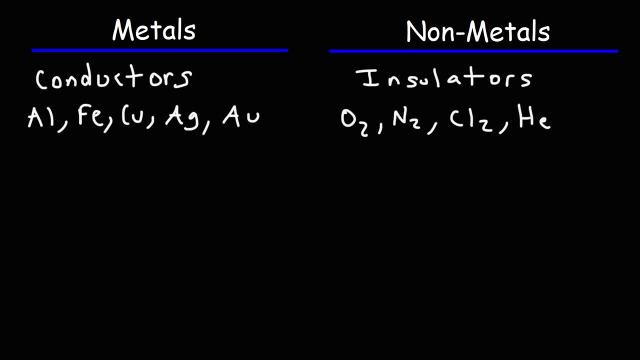 Think of helium gas. perhaps you've seen those helium balloons that rises up. Sulfur is a non-metal. none of those conduct electricity. now metals: they tend to be very shiny. they have a metallic luster. nonmetals are usually dull. they don't have that same metallic luster that metals do- most metals. 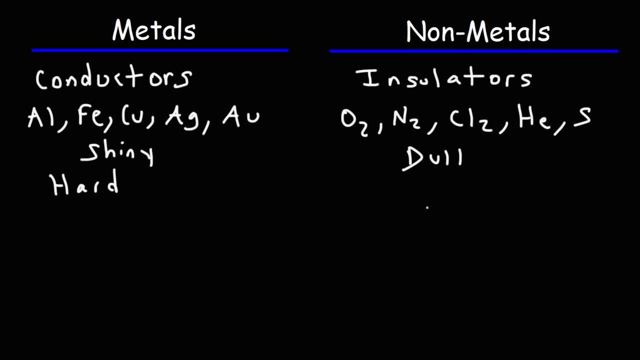 tend to be hard. they don't break easily. nonmetals: the majority of them are usually brittle in their solid form. now there are some metals that are soft, particularly the alkali metals like sodium and potassium. you can cut them with a knife, but the majority of metals they tend to be hard. now 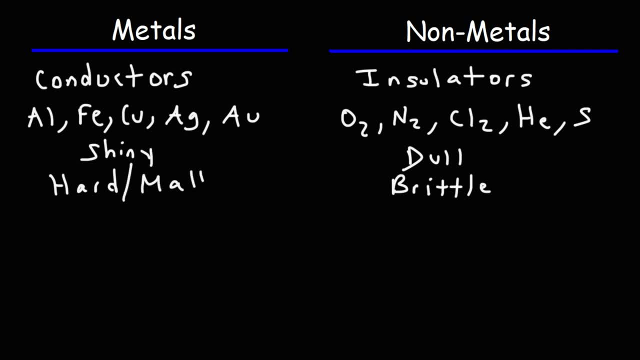 metals have another property: they're also malleable. this means that they can be hammered into flat sheets. metals are also ductile. they can be pulled or drawn into wires. now metals have another property. most metals are reducing agents- you reducing agents. they like to give away electrons. 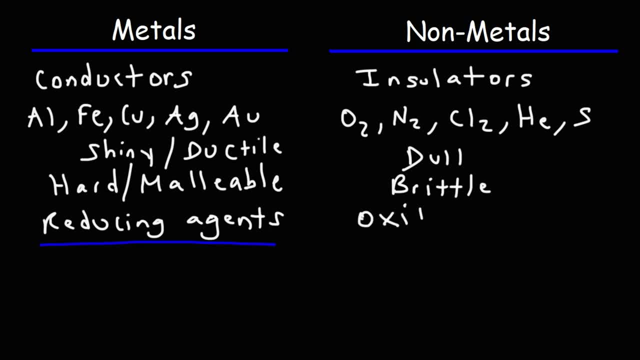 nonmetals tend to be oxidizing agents. think of the word oxygen oxidizing agents. they like to take electrons as opposed to give away electrons. so here's a reaction that can illustrate this: aluminum gives away its three valence electrons, it will form a 3 plus charge or positive 3 charge. another. 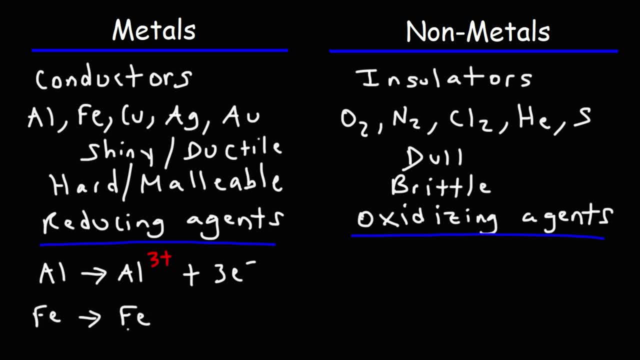 example is iron metal. when iron metal gives away two electrons, it will form the Fe2 plus ion. so, as you can see, metals are reducing agents. they like to give away electrons and in the process of of doing so, they will form positively charged ions known as cations. nonmetals are the opposite. 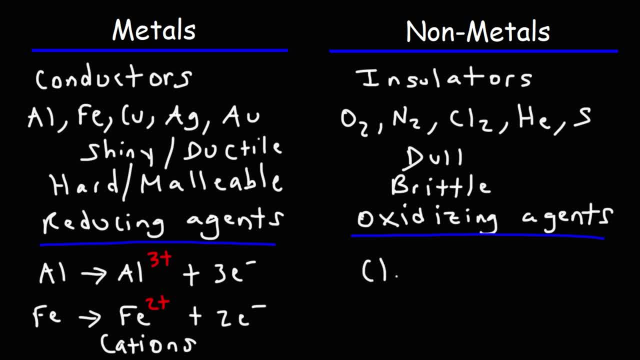 they like to take electrons. so chlorine gas is an oxidizing agent. when it takes two electrons it's going to form an ion with a negative charge, and the same is true for oxygen. but oxygen will form ions with a negative 2 or 2 minus charge, and negatively charged ions are 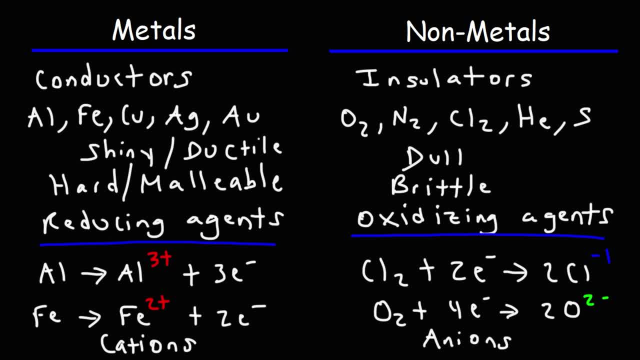 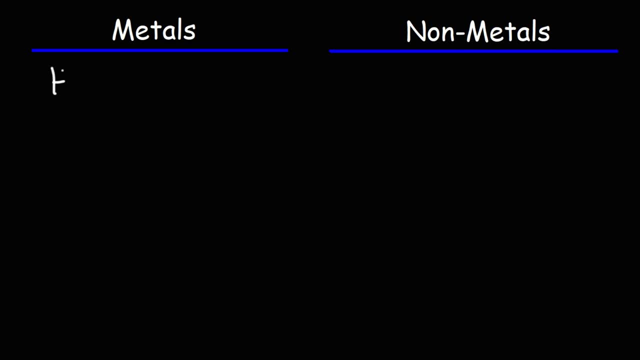 known as anions, so metals tend to form cations. nonmetals tend to form anions. metals tend to have relatively high melting points and boiling points. nonmetals tend to have low melting and boiling points compared to metals. calcium, for instance, has a melting point of 842 and a boiling point of 1484 degrees celsius oxygen on. 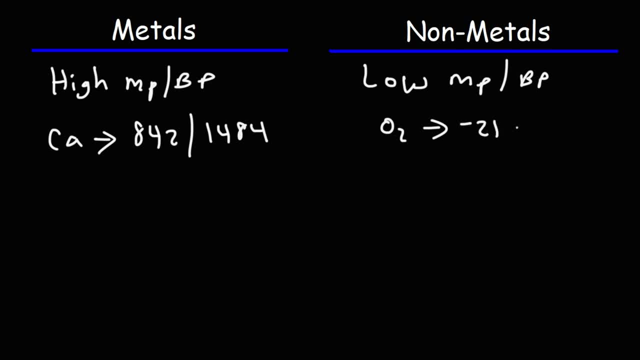 the other hand, has a melting point of negative 219 degrees celsius and a boiling point of negative 183. so most nonmetals. they tend to have low melting points and boiling points, whereas metals usually have much higher melting points and boiling points. but there are exceptions. for instance, sodium has a relatively low melting point. 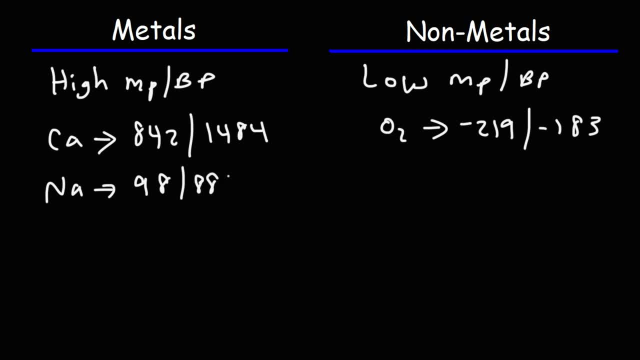 of 98.. its boiling point is pretty high: 883.. sulfur has a higher melting point than sodium. its melting point is 115. its boiling point is 445, but this is low relative to calcium tungsten has an extremely high melting point: 3422. its boiling point is 5930. iodine is another.